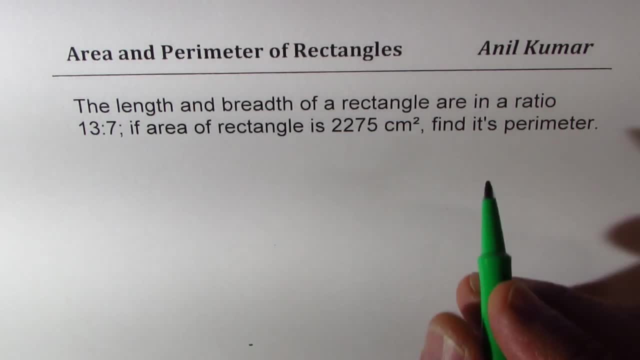 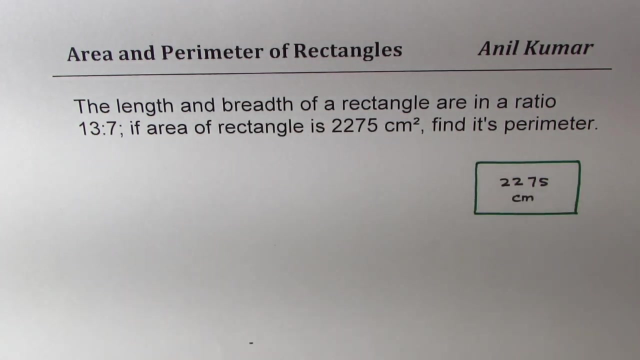 square find its perimeter. So let's sketch one rectangle here whose area is given to us as 20 to 75 centimeter square. Now, when we say that the ratio of length and breadth is 13 is to 7, it means what? So we are saying? ratio of length and breadth? 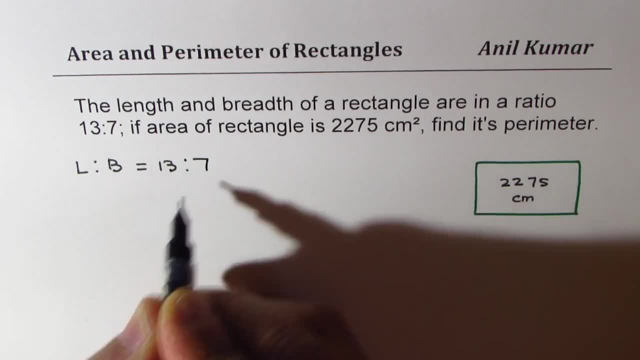 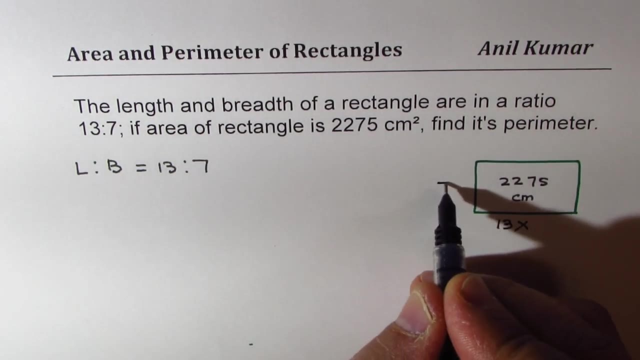 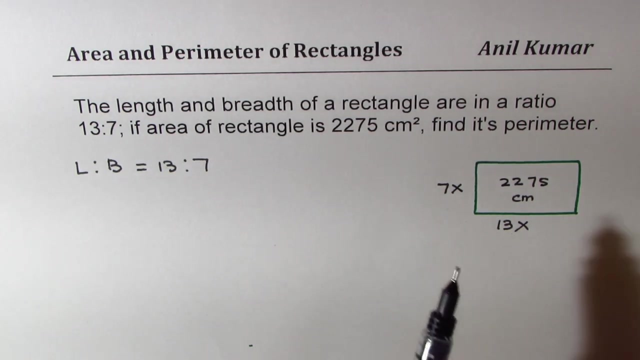 is equal to 13 is to 7.. That means it is 13 times something and 7 times something, right, So that is a constant. So that means it could be 13 times x, right, And 7 times x. So that is how we relate ratio with an algebraic expression. right To say 13 times x is equal to 7.. 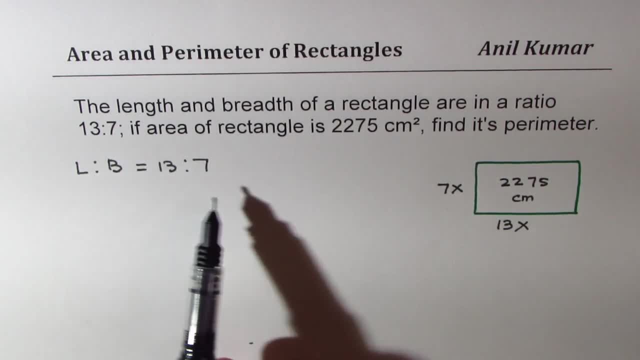 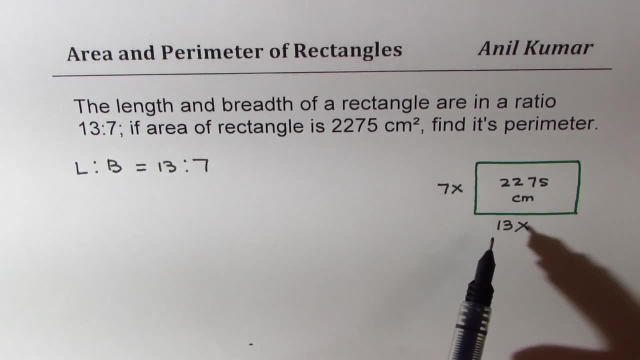 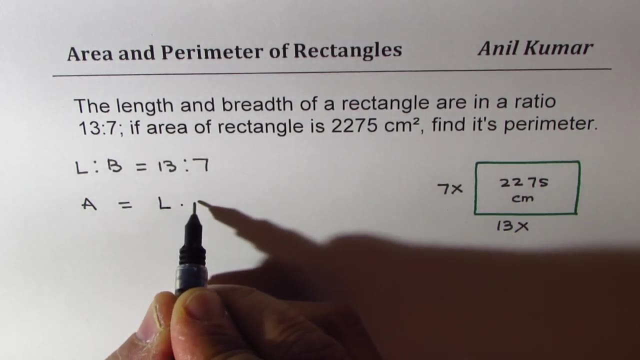 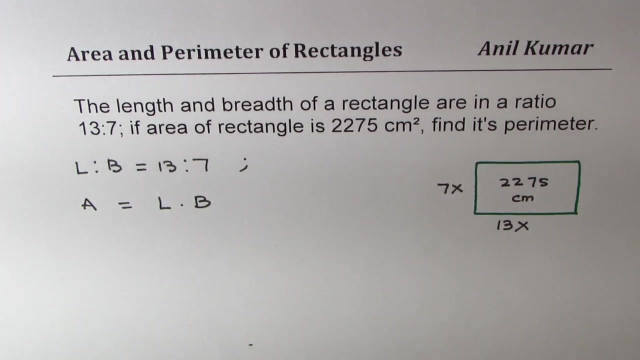 times something right. It could be times 2 x 3 x, 4 x 5 or whatever. So that is the relation right Now. from here the question becomes much simpler. So what is area equals to? So area will be equal to length times breadth Now, since we are taking length as 13x, so we have 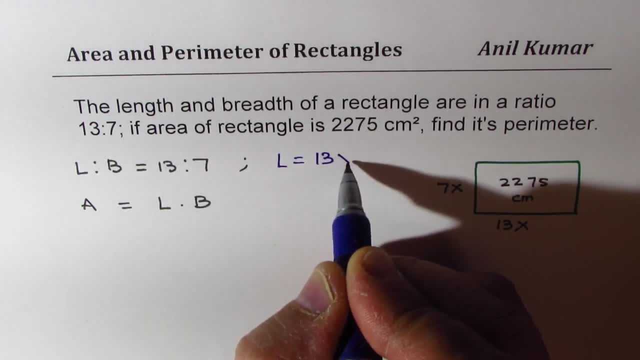 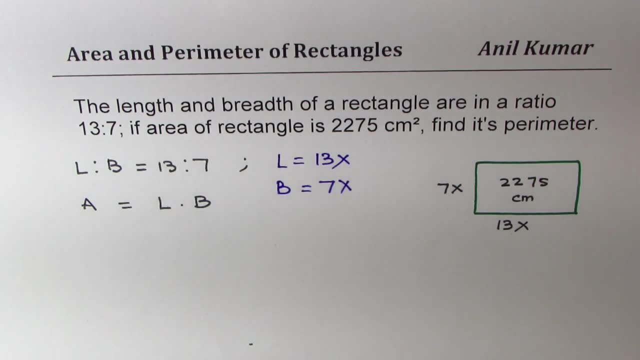 assumed that length is a multiple of 13, so it is 13x and the breadth is 7x. we'll substitute these values here and we are already. given that area is equals to 2275. right units are in centimeter square for area. so writing these values, we get. 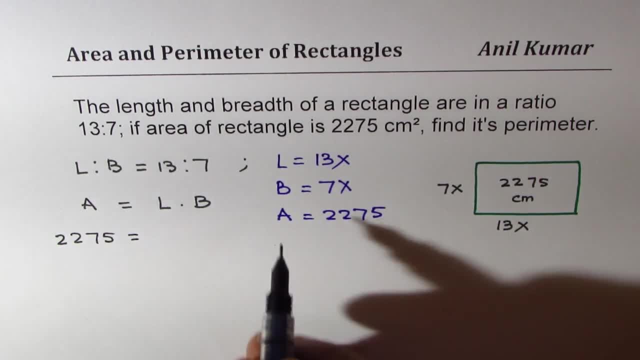 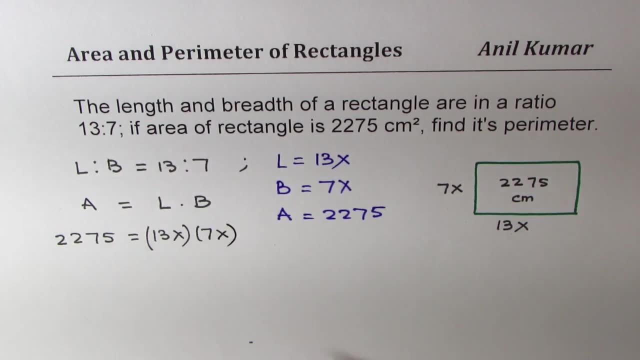 2275 for area equals to 13x times 7x. so 13 times 7 and x. so that gives you you could multiply now, or we could divide and then multiply, right. so so that gives you 13 times 7 times x square. 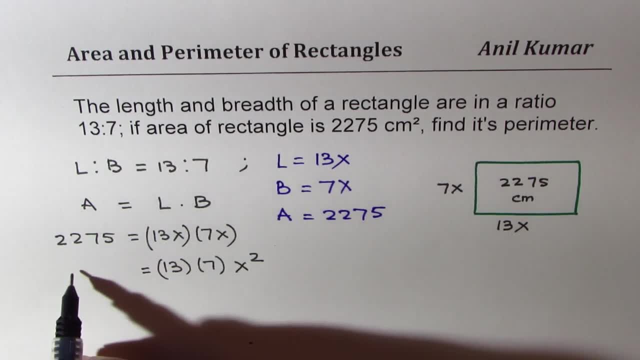 so when you multiply x and x, you get x square, and on this side we have 2275. now to find x, the constant ratio, we need to divide by 13 and 7, the left side. so we get 2275 divided by 13 times 7, right, and this is equal to x square. so let's put a dot here. 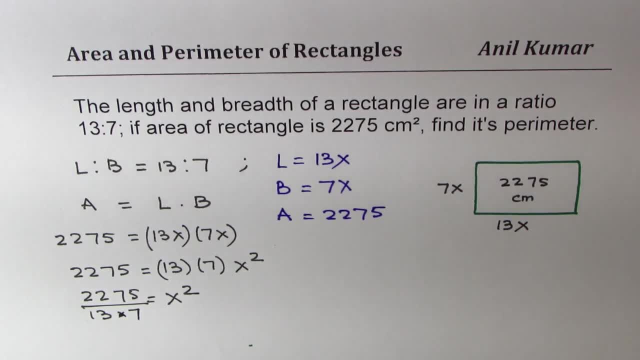 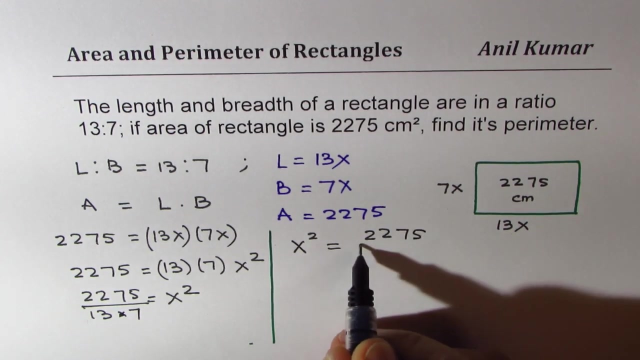 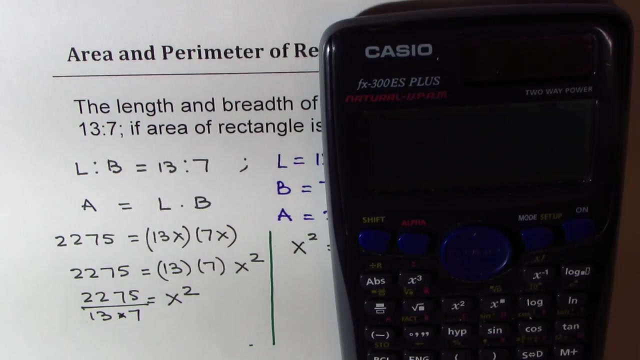 now you need to simplify this. you can also use calculator at this point to find this answer. so either way, you could do it right. so let's use calculator and find this answer. so what we have here is basically: x square equals to 2275 divided by 7 times 13, which is 91. so when you use calculator, you get 2275 divided by. 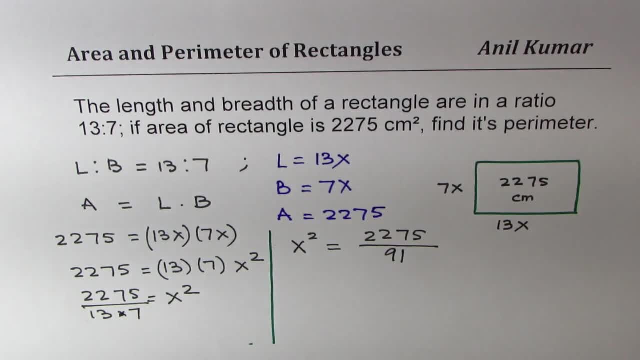 by 91 equals to 25, right, So you get x square equals to 25.. So if x square is 25, then x is square root of 25, which is equal to 5.. Now this question could have been done. 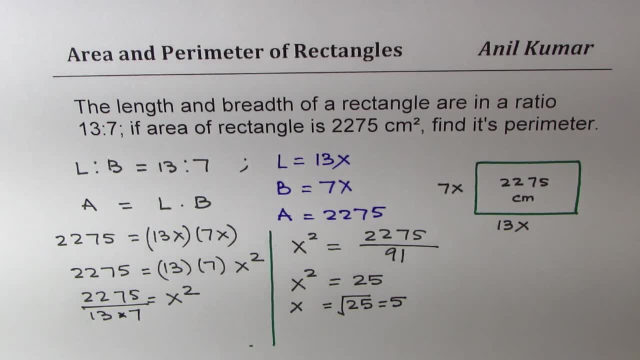 without calculator, also right Now. so x is 5.. Now can you write down the answer. I think it's clear. We have: length equals to 5 times 13,, right? So length is you can write 13 times 5,, right, which is 65, units being centimeters, and the breadth is 7 times. 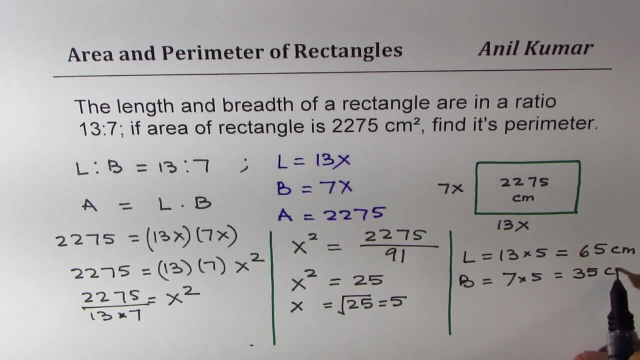 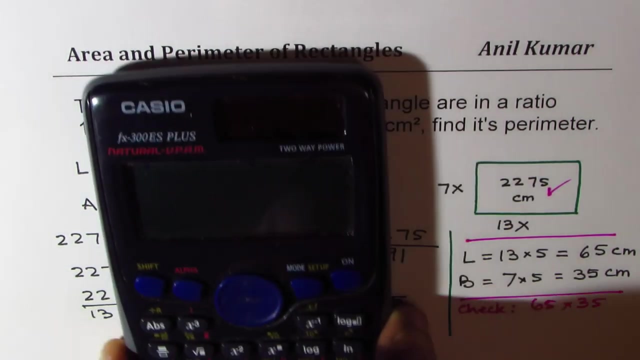 5, which is 35 centimeters, correct? So that becomes the solution for the given question. Now it's a good idea to check. So if you multiply 65 with 35, do you get this? That is what check is, So there is no harm doing it, So let's do it. We have 65 times 35,. 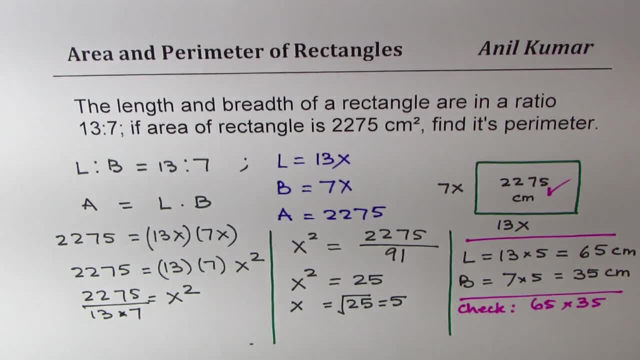 and we do get 2275.. Does it make sense to you? So that is how these questions can be solved. Feel free to write your comments and share your views. I hope you like the video. Thanks for watching and all the best.